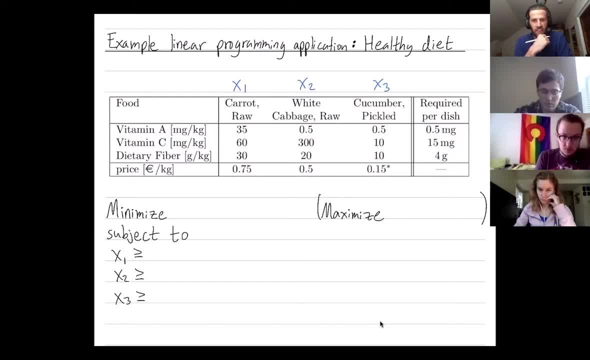 Gardner book. So we run a restaurant and we serve burgers, hot dogs, not so healthy stuff- And we got a decree that we need to start making our meals up to certain standards. So every time we serve a full course meal we have to have so much. 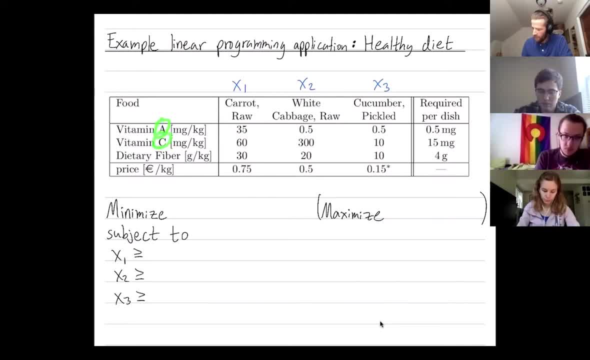 vitamin A, vitamin C and dietary fiber. Otherwise the Colorado Health Board of Education is going to clamp down on us. So every dish we serve we need at least 0.5 milligrams of vitamin A, 15 milligrams of vitamin C and four grams of fiber. 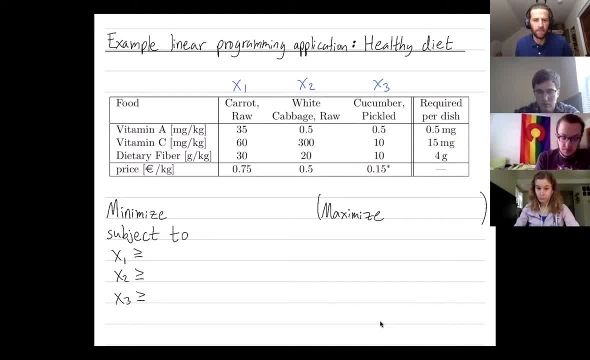 Per kilogram Or per dish, I guess. Okay, so we serve hot dogs, hamburgers, you know those are the top sellers. But what we're going to do is we're going to make a mash of vegetables. It's going to be a mash containing carrots and cabbage and cucumbers. 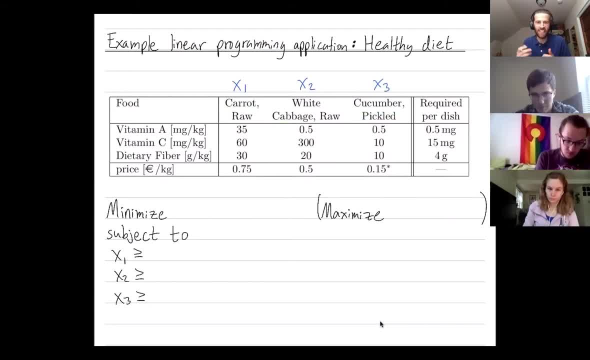 Okay, and we're going to make like a little salad or a mash of carrots, cabbage and cucumbers And we're going to serve it as a side dish With every hamburger and hot dog meal that people order. Okay, and our question is: well, okay, this is not good, But we're cheapskates And we want to combine carrots and cabbage and cucumbers in the cheapest way to get up to the required amount of vitamin A, C and fiber. Okay, 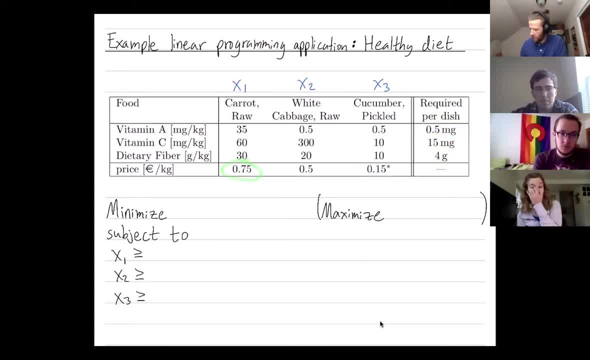 But we don't. we don't want to pay too much. So this is just an example. Okay, This is how much it costs for carrots and cabbage and cucumbers, And we don't want to pay pay too much. Maybe it's because we're cheapskates, But maybe the better reason is the leftover money we get to donate to to. yeah, Jack is laughing at me. Oh, sorry, Jack, I just mentioned your name on YouTube. 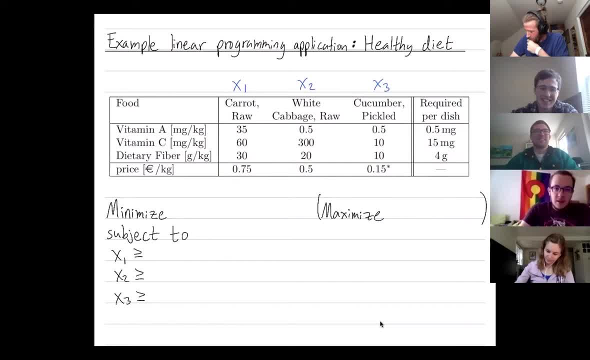 All right, Let's see. Okay, so right Here we've listed how much vitamin A carrots have, So 35 milligrams per kilogram, And this is how much vitamin C and how much fiber they have. So what is our optimization problem? We're trying to minimize the cost, So let's first choose our variables. X1 is going to be the kilograms or grams of carrots. 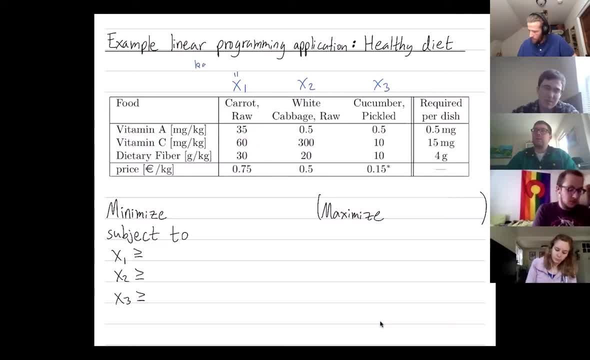 And X2 is going to be your kilograms of cabbage And X3 is going to be the kilograms of cucumber. We're trying to minimize cost. So how do I get the cost? Well, I have to pay 0.75 pounds for every unit of carrots. 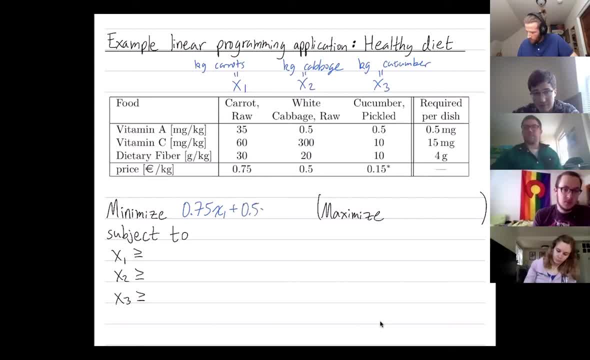 Plus 0.5 pounds for every unit of cabbage Pounds. pounds are sorry, pounds is not a unit of weight here, Pounds are, or maybe these are euros? Okay, Yeah, We have to pay 0.75 euros for every unit of carrots. We have to pay 0.5 euros for every unit of cabbage And we have to pay. 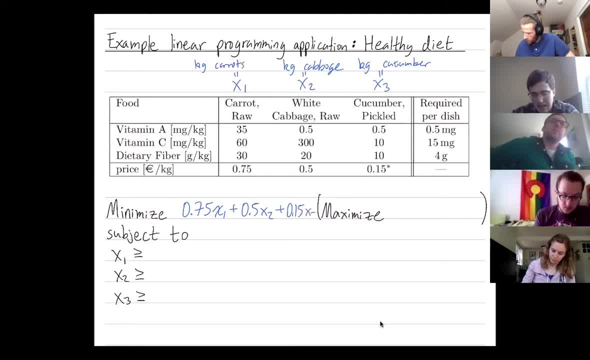 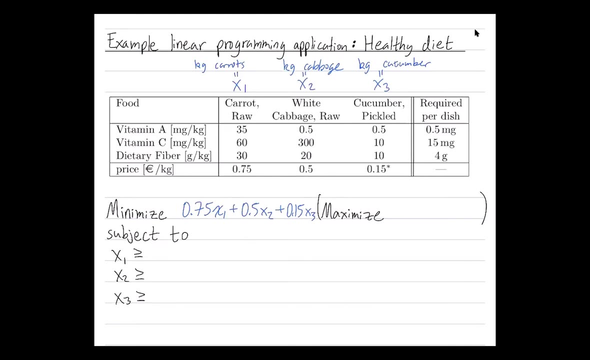 0.15 Euros for every yield of nuts of cucumber. We're trying to minimize costs. Later in this class we're going to essentially recast every optimization problem as a maximization problem, and you can do that If we instead wanted. 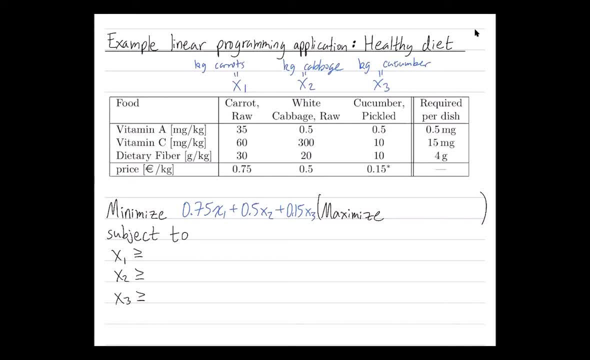 to maximize something. just multiply this function by negative 1, and then we're trying to maximize it. Okay, but we have these constraints. We need to serve folks a healthy vegetable side dish, so our constraints are well. first, we can't serve them a negative amount of carrots or a negative amount. 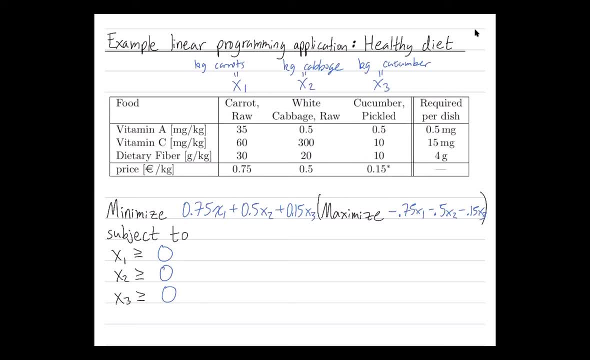 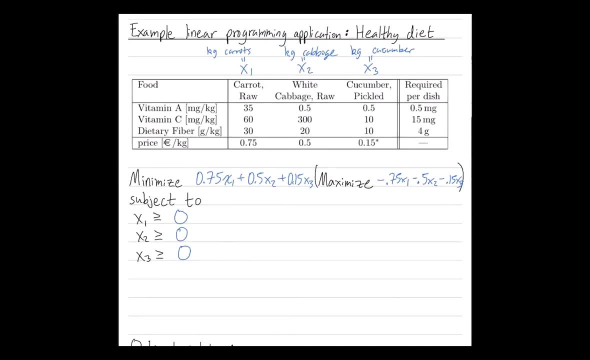 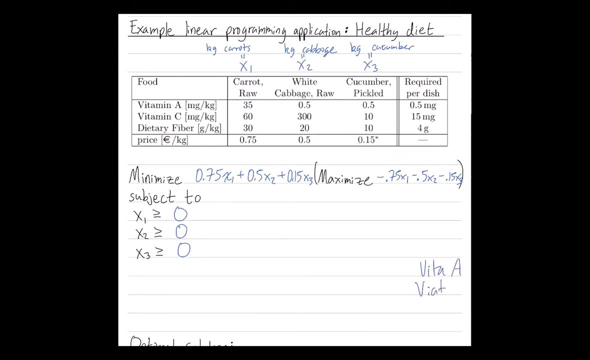 of cabbage or a negative amount of cucumber. That would just be unethical, impossible. Also, we sort of have a vitamin A constraint. We need to serve up enough Vitamin A. We also have a vitamin C constraint and we also have a fiber constraint. Okay, so what is the vitamin A? 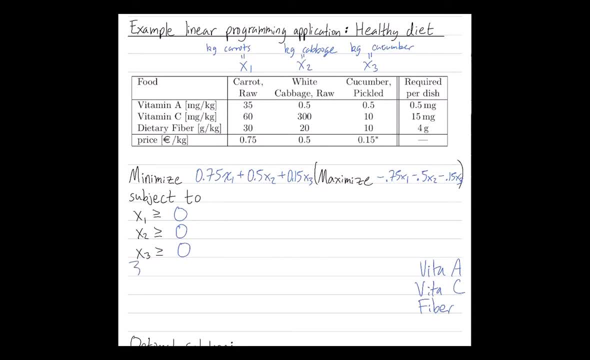 constraint? Well, thirty-five times the amount of carrots, plus point five times the amount of cabbage and cabbage, plus point three times the amount of cabbage and cabbage. So it's a little bit more complex. So there's one thing about vitamin A constraint is that if you're 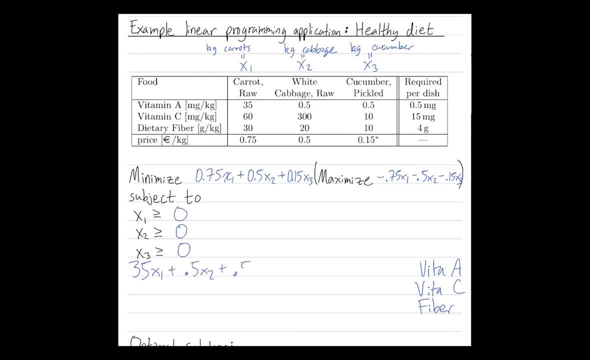 amount of cabbage plus 0.5 times the amount of pickles has to be at least the required amount of vitamin A, And then our vitamin C constraint is 60 times the amount of carrots, plus 300 times the amount of cabbage, plus 10 times the. 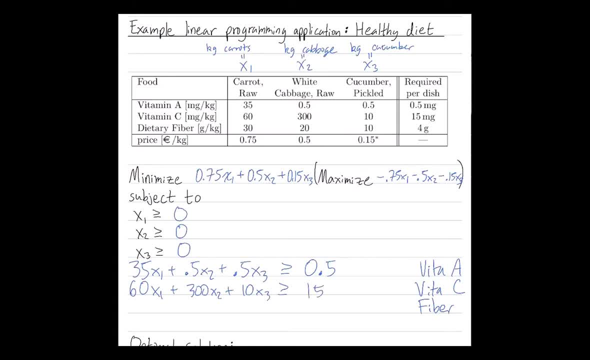 amount of cucumbers has to be at least our 15 milligrams of vitamin C. And then our fiber constraint is that 30 times the amount of carrots plus 20 times the amount of cabbage, plus 10 times the amount of cucumbers has to be at least. 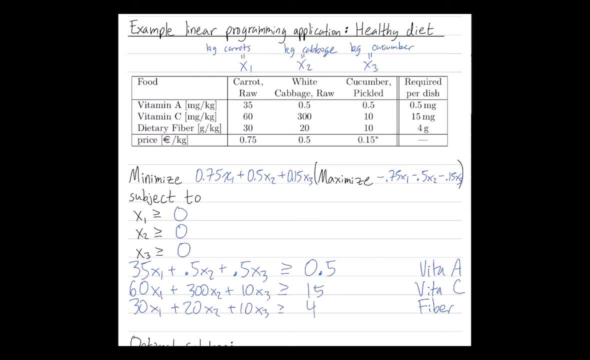 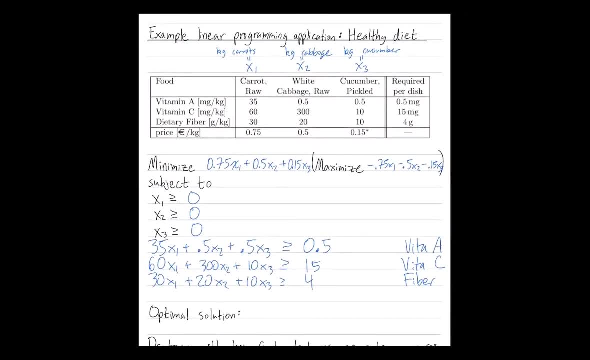 our 4 grams of fiber. Questions so far. We won't. we won't solve this today, but I'll tell you the solution. The solution is we're gonna write these amounts of carrots, cabbage and cucumbers in grams instead of kilograms, but whatever. So the optimal solution is 9.5 grams of. 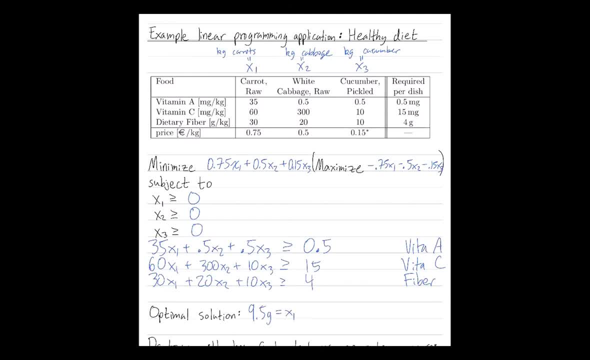 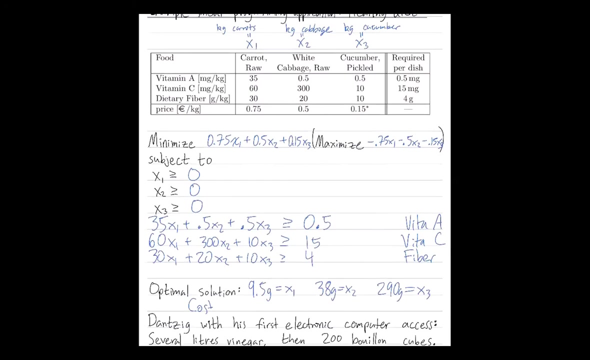 carrots and cabbage will be 38 grams And pickled cucumbers will be 290 grams per dish, And the cost of this is 0.07 euros. So we're doing so pretty cheaply. Those numbers are all rounded. 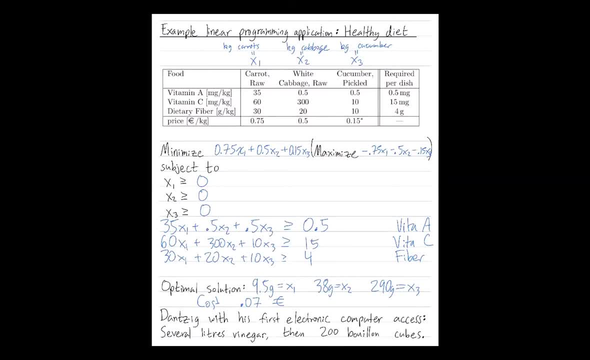 One thing I should say is that this solution might not satisfy other priorities or constraints you might have. You might come along and say, wow, that's way too much cabbage. Nobody's gonna like this dish, And so what's often done is people will solve one linear program. find out, they really. 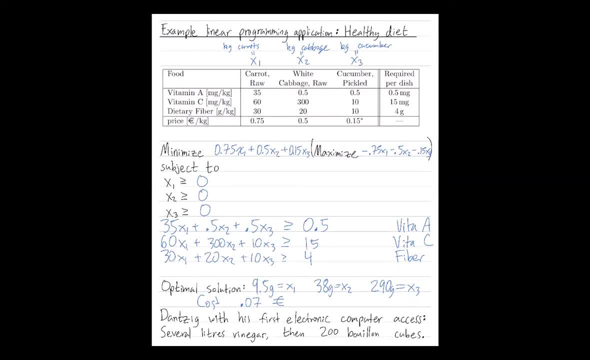 have more constraints than they told the algorithm at first and then just add in an extra constraint. So you might come along here and add in an extra constraint, say you know, maybe I only reasonably expect to be able to sell my food if I have at most. 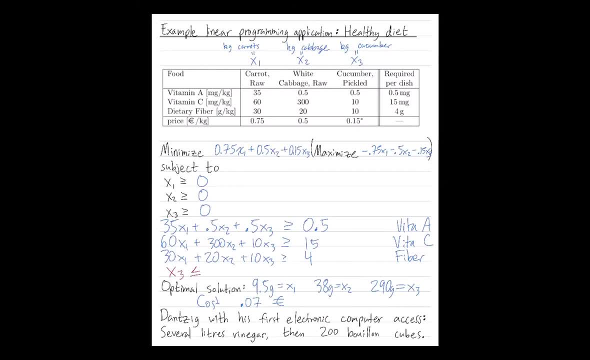 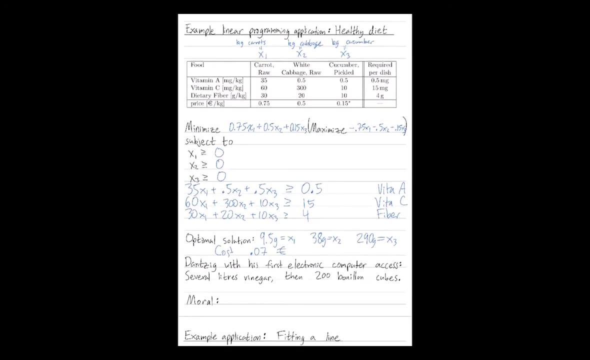 you know, 100 grams of cabbage, So you add in an extra constraint. This actually sort of happened in the following sense. So George Danzig is one of the heroes of this class. He invented the simplex algorithm and he did so, you know, when it was hard to get access to computers, But once he got, 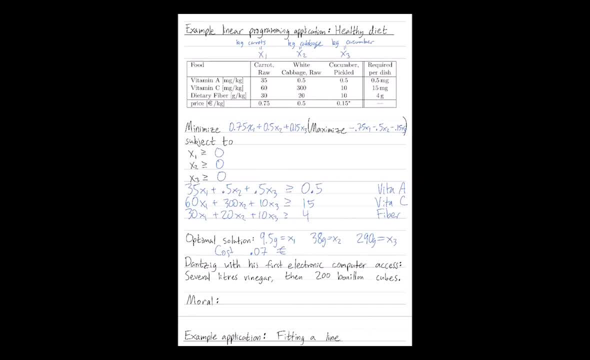 computer access. he tried to optimize his diet So he plugged in all of the foods he ate and he plugged in these nutrition constraints and he plugged in the prices and he sort of said: how much do I need to spend if I want to live healthfully? The first time he ran this algorithm 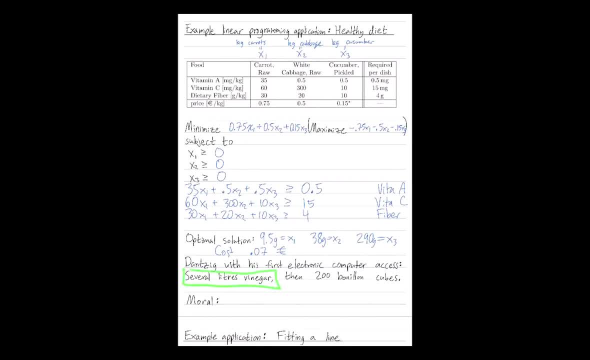 the optimization was done. And he did that because he wanted to optimize his diet. And he did that because the optimization problem said: hey, George, you should drink seven liters of vinegar a day. That should be your diet. And he said, huh, that's not so appealing to me for other reasons. 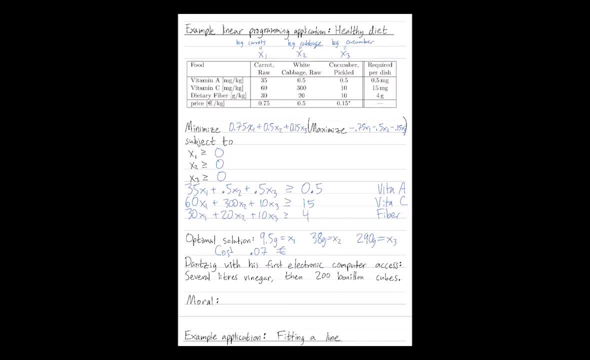 And it's probably not healthy. You know, he probably didn't correctly model all the health constraints, So he added in a constraint: Okay, let's keep my vinegar amount below a reasonable level. And then the next time he ran this program the computer told him to eat 200 bouillon cubes. 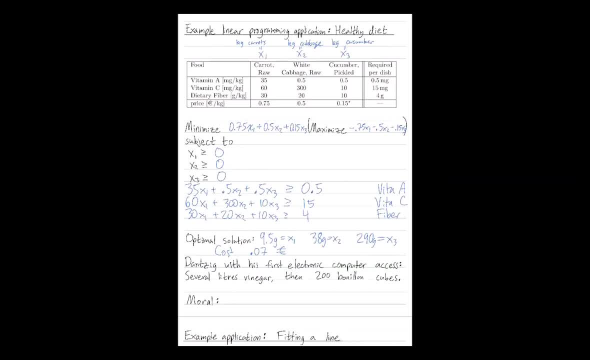 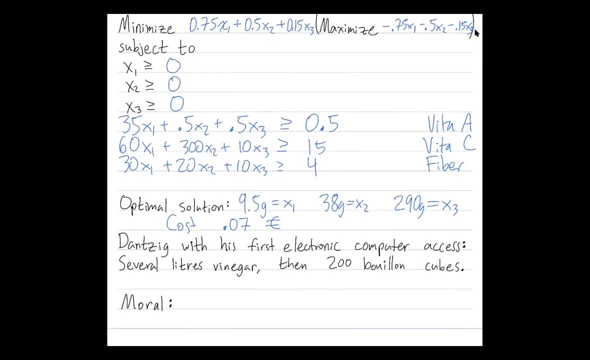 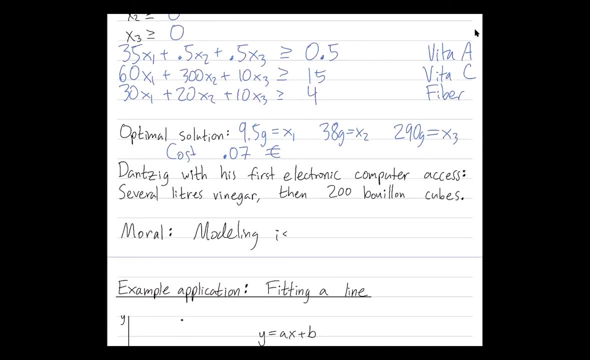 a day, which is also pretty hilarious- And he said, no, I don't want to eat 200 bouillon cubes a day. So he kept adding on more constraints. So the moral of this is like modeling is hard And you should not be super confident that you can model the real world by mathematics, I mean.